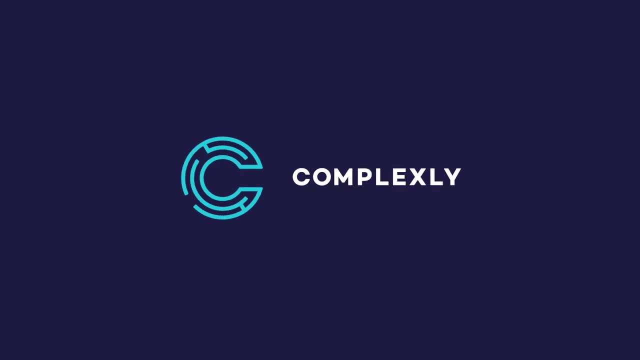 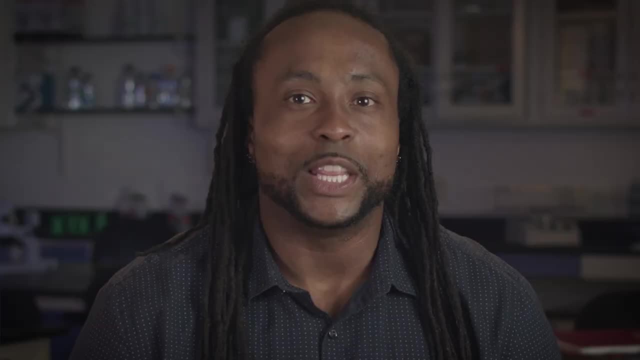 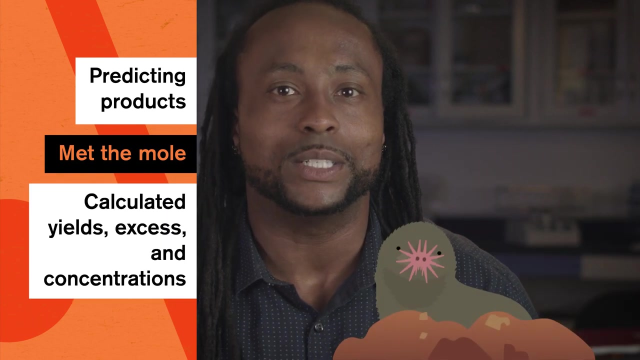 We said at the beginning of this series that everyone is capable of being great at chemistry using motivation and confidence. And look where that combination has gotten us so far. We mastered predicting products, met the mole and calculated yields, excess and concentrations. 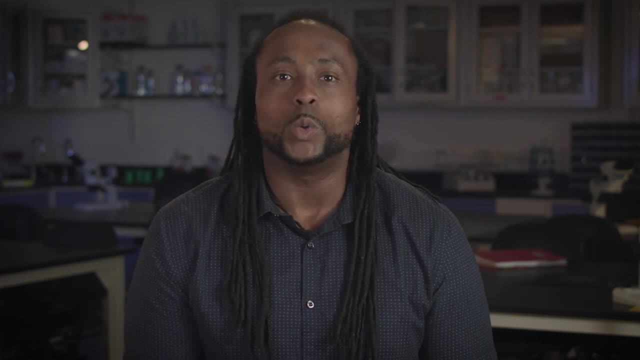 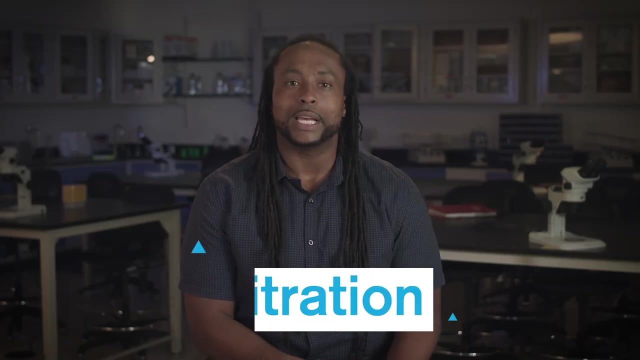 And now that we're familiar with all of that and acid-base reactions, we'll dig into the details of strong and weak acids and bases, including buffers, and talk about why they're important. We'll also go through a titration or the neutralization of an acid and base in reaction. 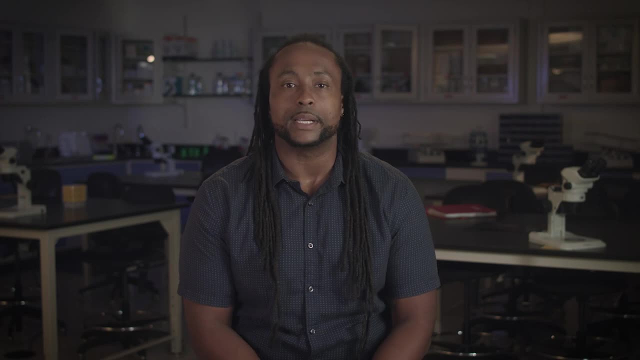 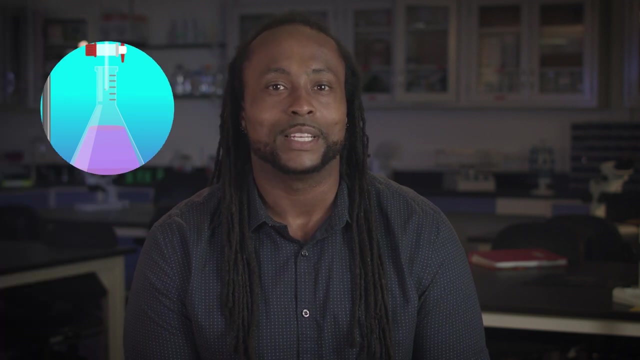 because it's a great way to visually show the changes the substances experience. Titrating acids and bases produces a cool colorful change, but there's far more going on inside that Erlenmeyer flask. We'll get into all that detail today in our final episode. 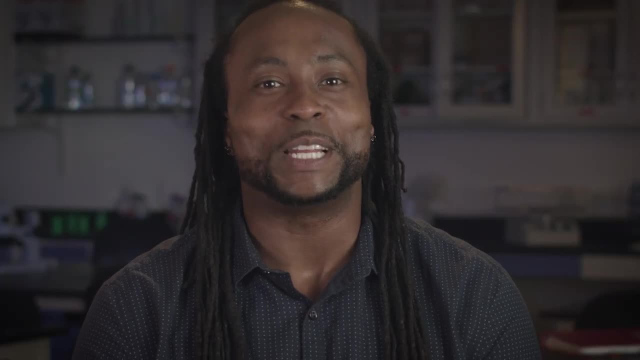 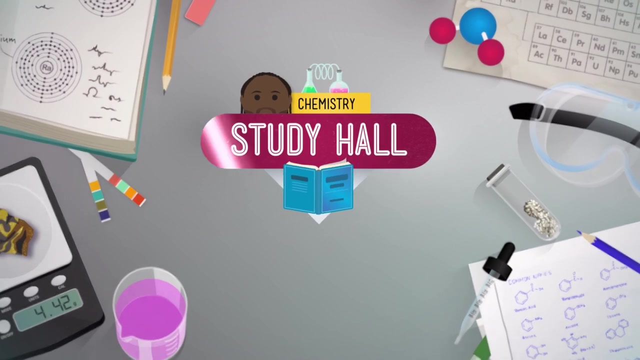 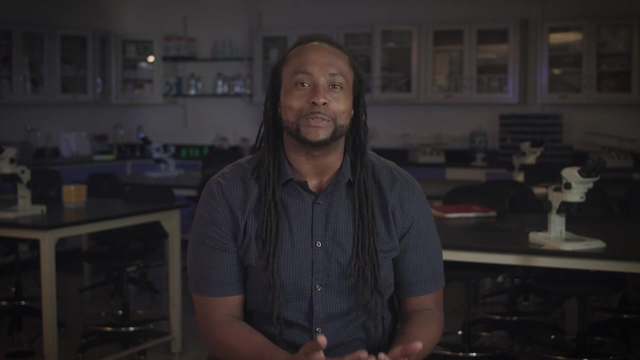 Hi, I'm Will Comar and welcome to our last episode of Study Hall Chemistry presented by Arizona State University and Crash Course. Let's dive in. Before we splash into any titrations, let's take a minute to go over some of the essential. 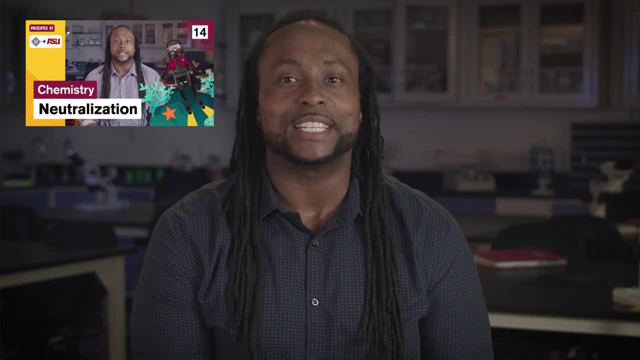 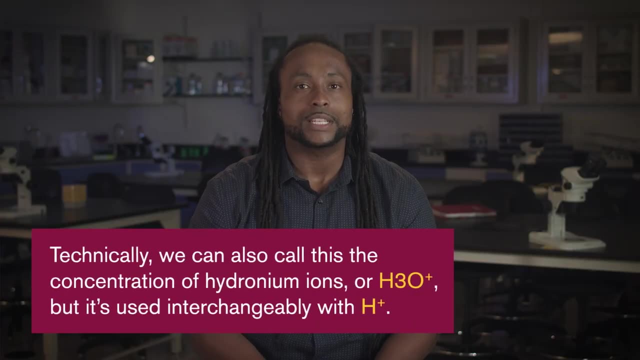 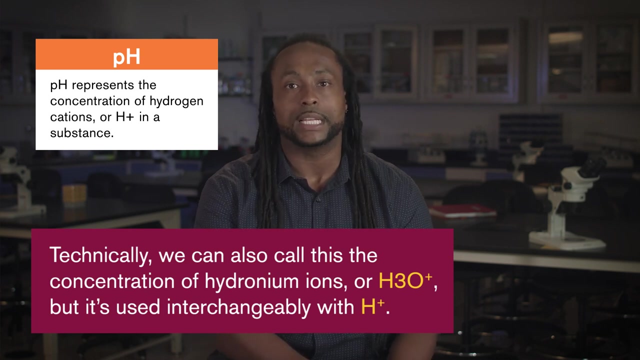 vocabulary first From last episode. you probably remember, acids have high H-plus concentrations and bases tend to have high concentrations of hydroxide or OH-. We show those concentrations in two terms. One is pH, which we covered last time. It represents the concentration of hydrogen cations, or H+, in a substance. The other is pOH- a. 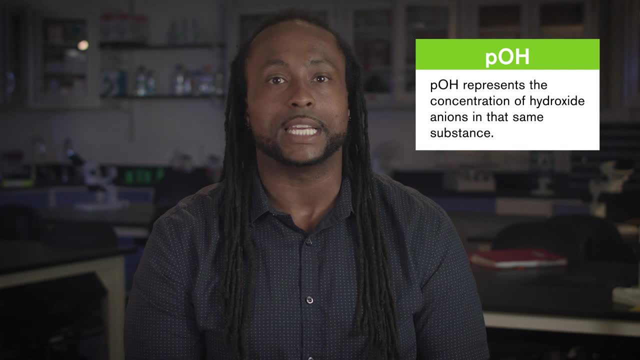 value that represents the concentration of hydrogen cations in a substance. The other is pOH, a value that represents the concentration of hydrogen cations in an individual substance of hydroxide anions in that same substance. Acids and bases have both a pH and a pOH. 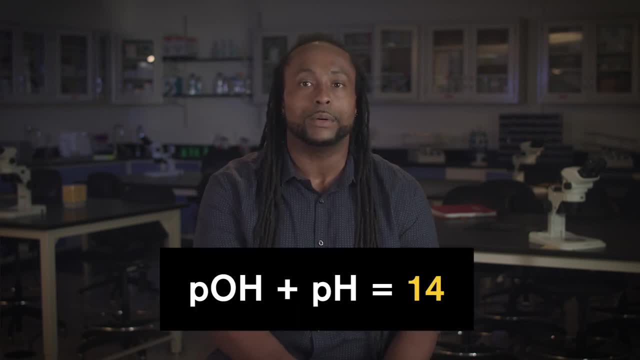 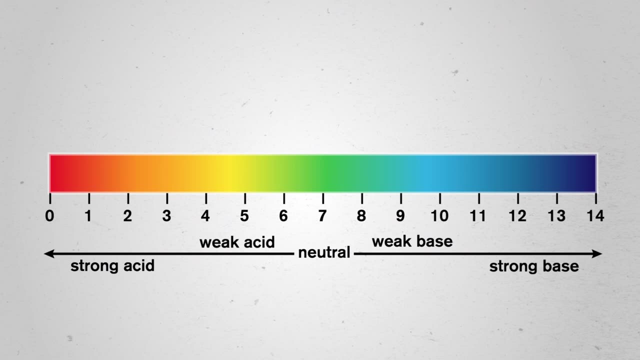 In fact, we usually represent the relationship between them, as pOH plus pH is equal to 14.. If we know the pH, we can find the pOH, and vice versa. The reason we can do this is because of what these scales actually look like. 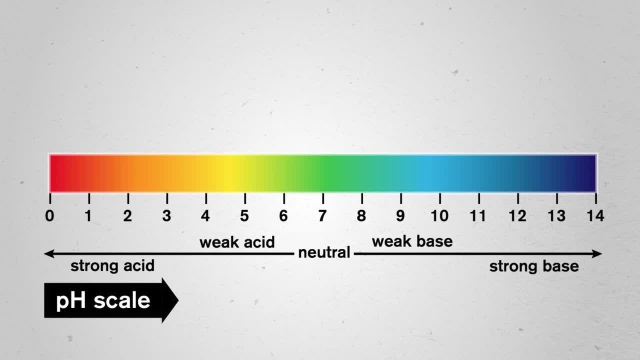 The pH scale is a visual representation of the strength of acids and bases on a scale from 0 to 14, with acids on the low end, bases on the high end and neutrality right in the middle, at 7.. The pOH scale is like the pH's mirror image. 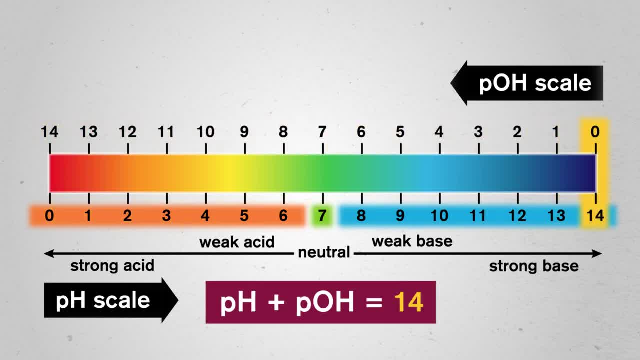 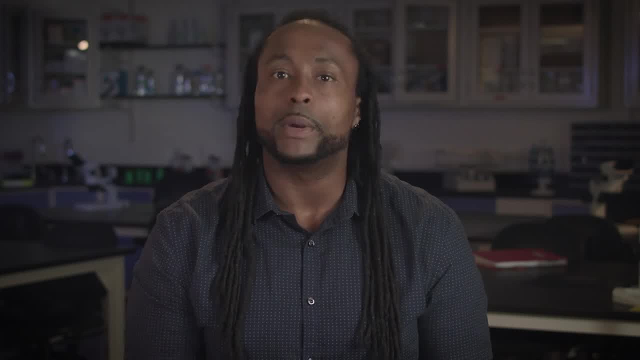 So when the pH is low, the pOH is high and they always add up to 14.. It might seem tricky at first to remember how a pH or pOH value relates to acids and bases, but we can use two rules to help us out. 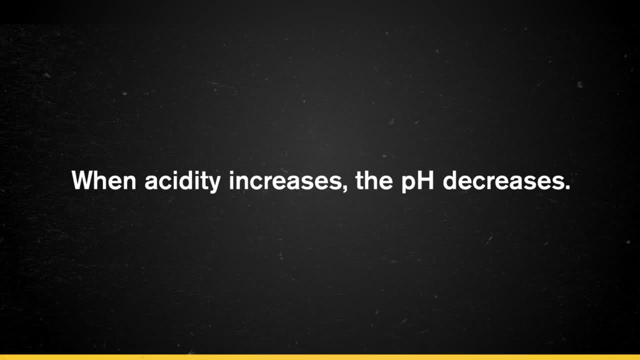 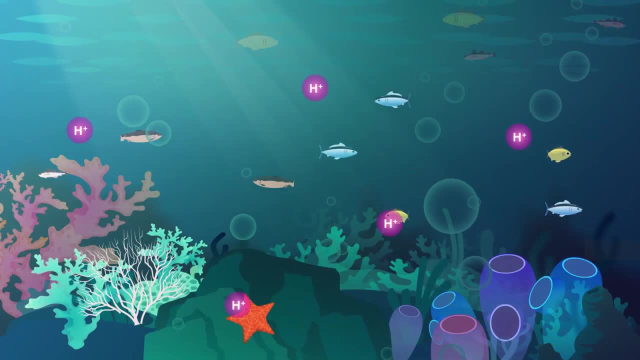 One, when acidity increases, the pH decreases. And two, when substances become more basic, the pOH decreases. For example, the pH of seawater is at a slightly basic 8.2.. If it becomes more acidic over time, the pH will decrease and move closer to the acidic. 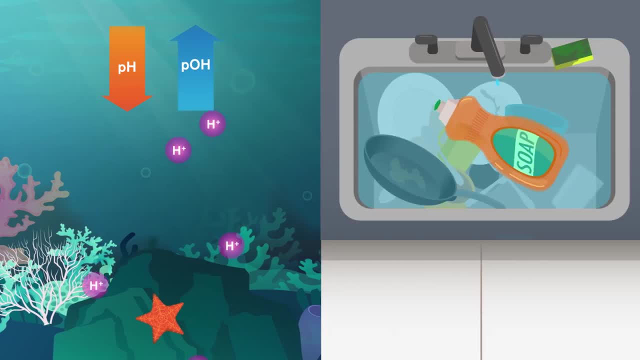 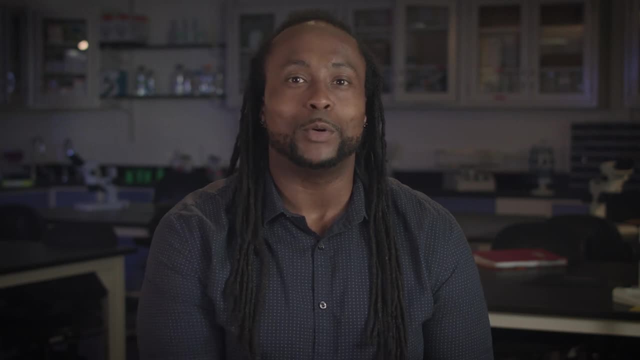 end of the pH scale, while its pOH increases, And adding soap to water makes it more basic, which increases the pH and decreases its pOH. pH and pOH represent the full spectrum of acids and bases, which means there are both strong and weak acids and bases. 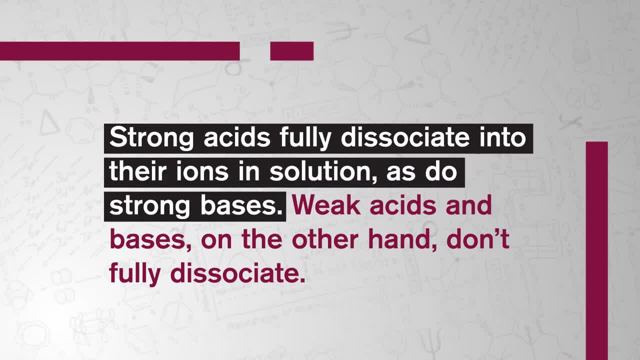 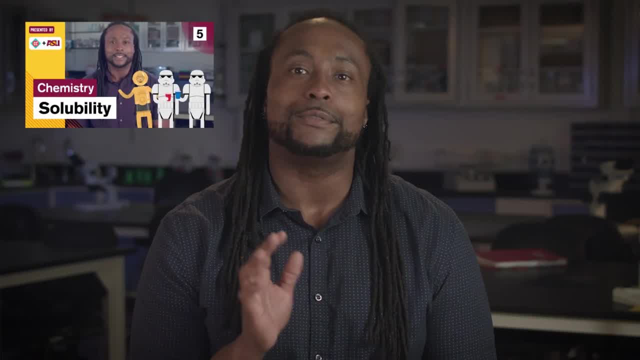 Strong acids fully dissociate into their ions and solution, as do strong bases. Weak acids and bases, on the other hand, don't fully dissociate. We defined dissociation back in episode 5, when we talked about solubility and ionic equations. 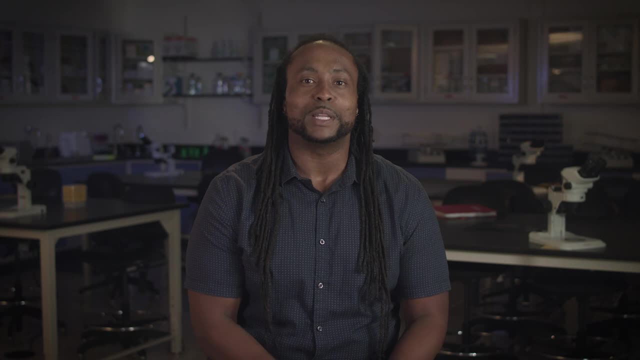 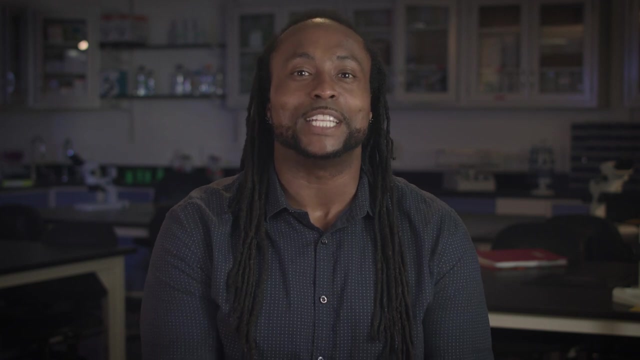 in case you need a refresher. Strong acids and bases are more well-known for playing the blockbuster roles in movies and dramatic reactions in your average lab experiment. But even though weak acids and bases tend to fly under the radar, they literally keep us alive. 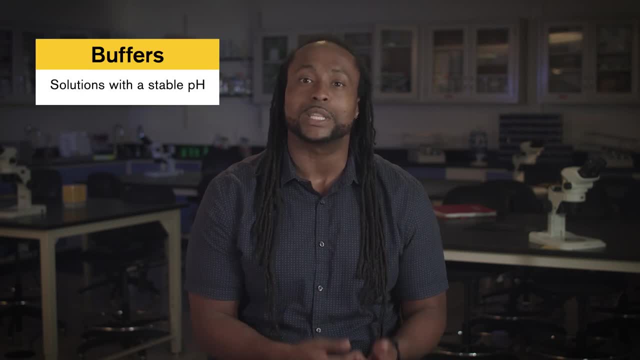 They play a huge part in creating aqueous buffers, which are solutions with a stable pH. In other words, they prevent pH from changing significantly. So we're going to talk about pOH and pOH in a little bit, But not significantly. when, in the presence of a strong acid or a base, 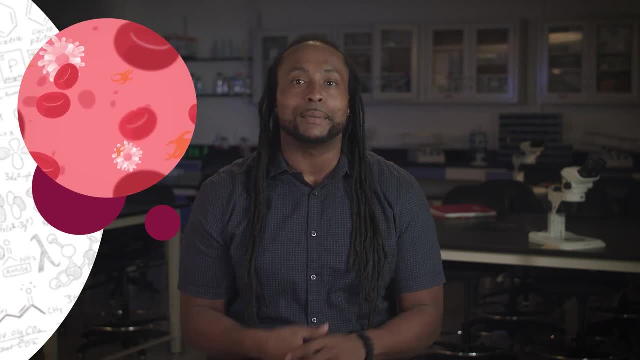 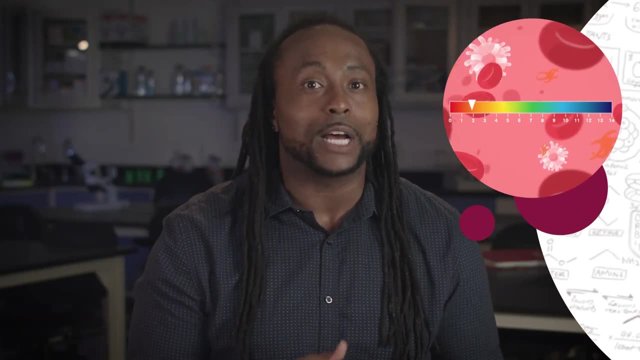 For example, our blood contains a buffer made from carbonic acid and a bicarbonate ion that maintains a narrow pH range. If we didn't have that buffer, our blood pH could rise or fall out of that healthy range, which could be deadly. 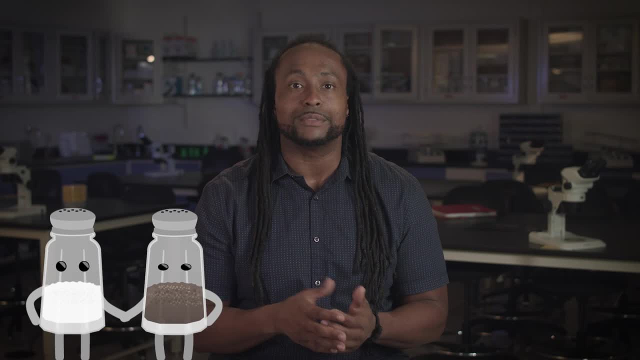 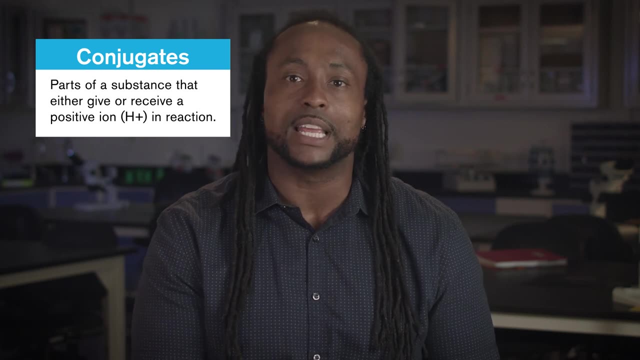 Buffers work in pairs, using teamwork, to prevent the pH of a solution from changing drastically, and it's all got to do with ions. Buffers require conjugates, which are the parts of substances that either give or receive a positive ion in reaction. 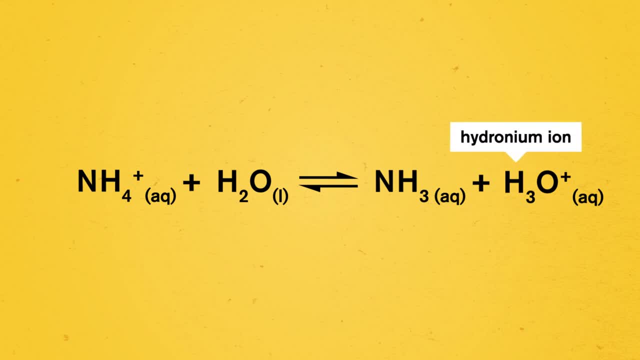 A conjugate acid is a weak acid that donates or loses its H plus ion. Ammonium is a conjugate acid because when in solution it donates an H plus ion to become ammonia, which is a weak base. Acetate is the conjugate base of acetic acid, since it receives the H plus ion from the 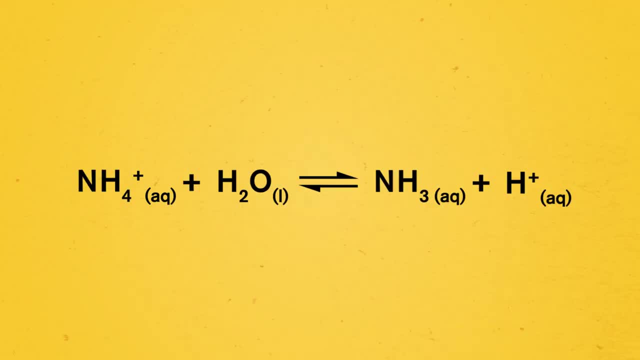 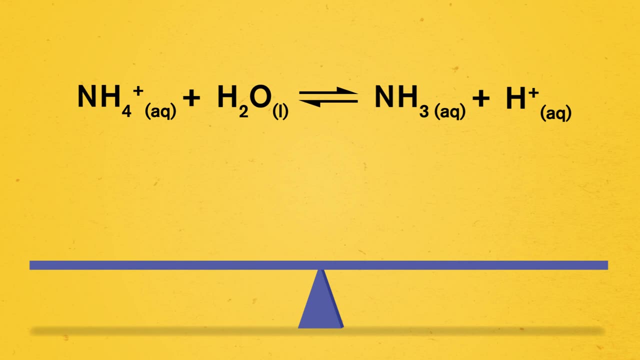 weak acid Conjugate reactions are reversible, so we could look at them going in either direction. It's like a seesaw or a tightrope. If we have a lot of H plus ions, for example ammonia would take them on to produce more. 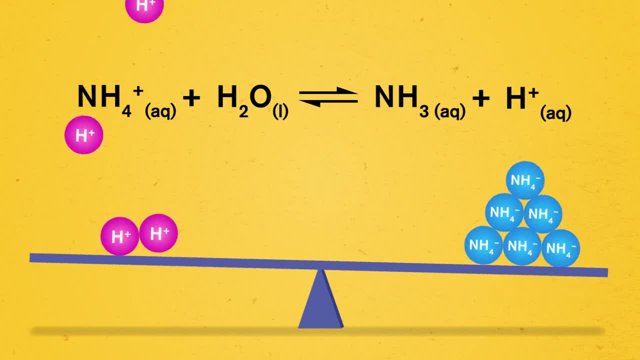 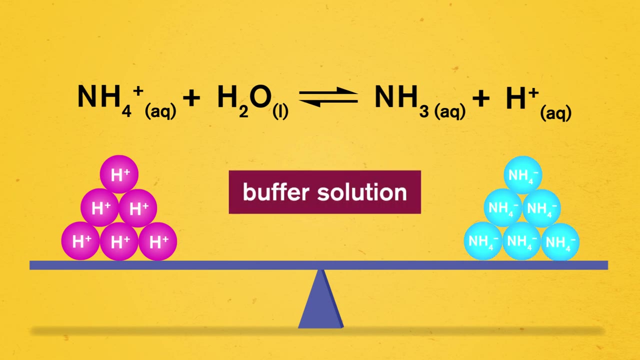 ammonium. If we have more ammonium, the reaction would donate its H plus ions back to the ammonia to maintain balance. So when a solution contains either a weak acid and its conjugate base or a weak base and its conjugate acid, this is called a buffer solution, which uses the conjugate ions to 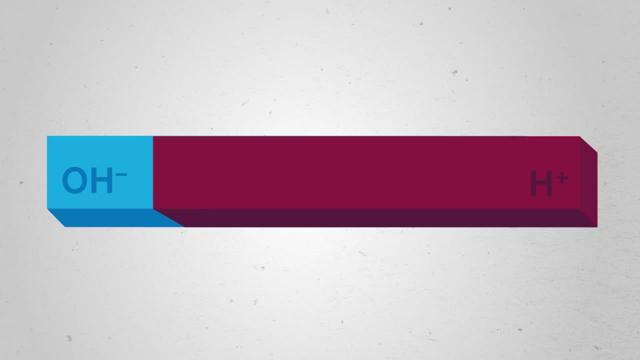 resist pH changes. The conjugate pairs do their balancing act. if something new goes into the solution and there's extra ions for them to deal with, Like if a strong acid gets added, that means we've increased the concentration of our H plus in our reaction. 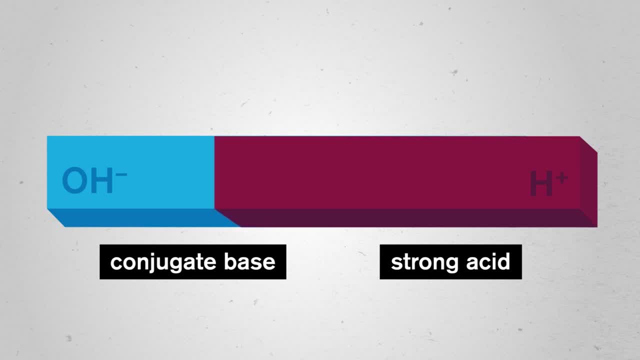 This disrupts the equilibrium and prompts the reaction to form more of the conjugate base in order for us to get back to equilibrium and maintain the solution's pH. If we added a strong base instead, that would push the equilibrium the opposite direction, prompting it to make more of the weak acid in order for balance to be restored. 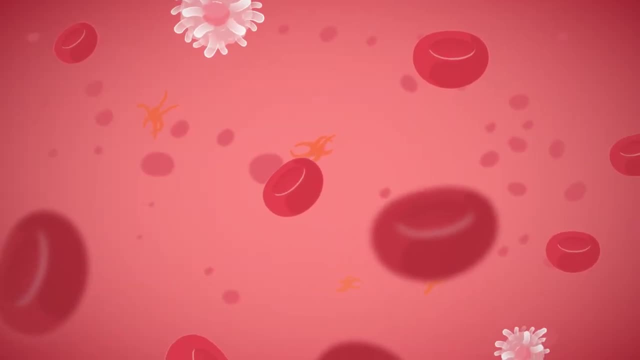 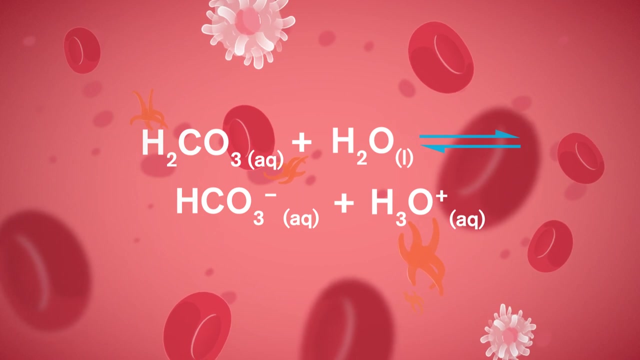 Buffers are best explained with an example, so let's talk a bit more about our blood. The human body is super complex but, simply stated, human blood is at equilibrium between bicarbonate and carbonic acid. This is a reversible buffer solution. 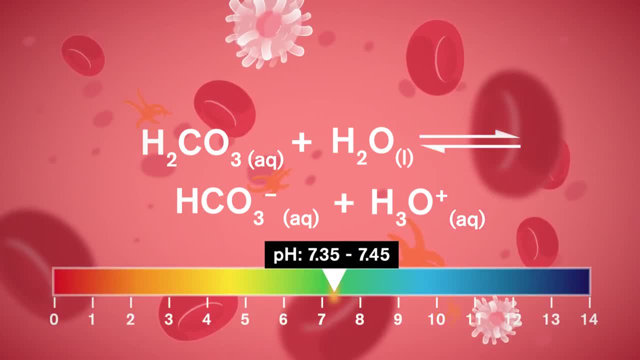 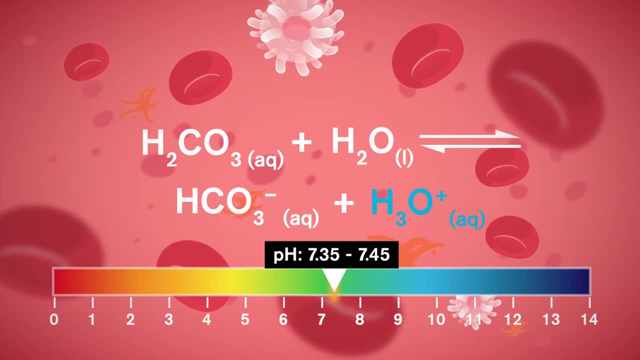 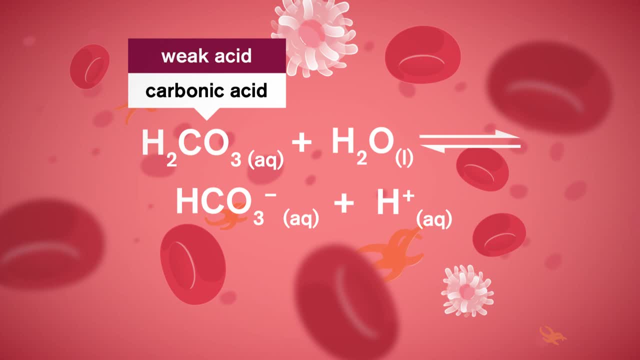 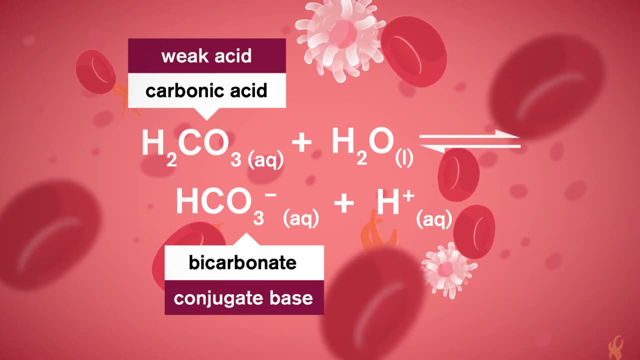 remember we call H plus. In this situation, carbonic acid is the weak acid and the bicarbonate is the conjugate base. Bicarbonate prevents acid form building up in the body and carbonic acid keeps the pH from getting too basic. 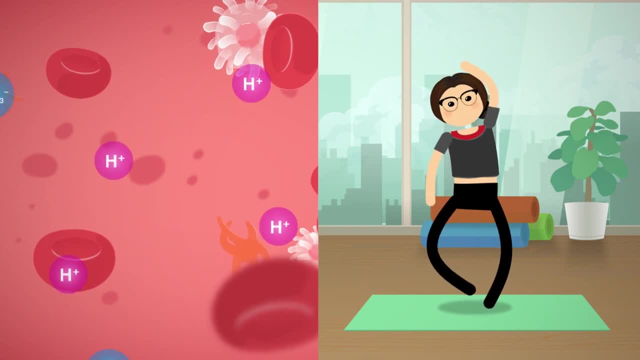 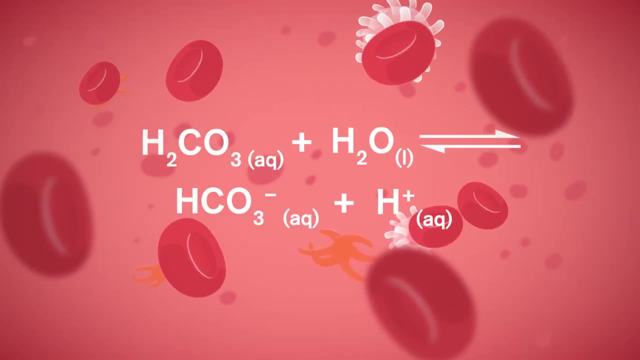 When we exercise, H plus ions accumulate in our blood, so our kidneys secrete bicarbonate to dual bond to it and produce carbonic acid acid which we breathe out through our lungs. On the other hand, if we don't have enough H+, our blood pH increases, so the body converts. 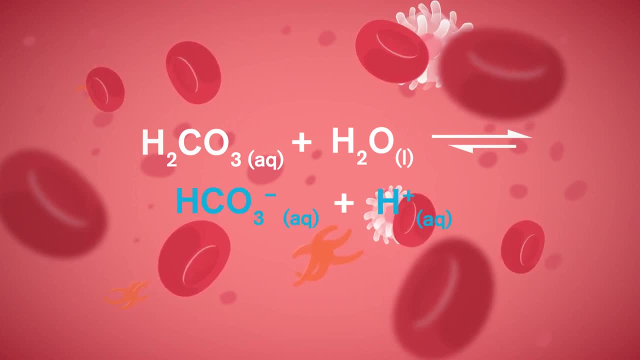 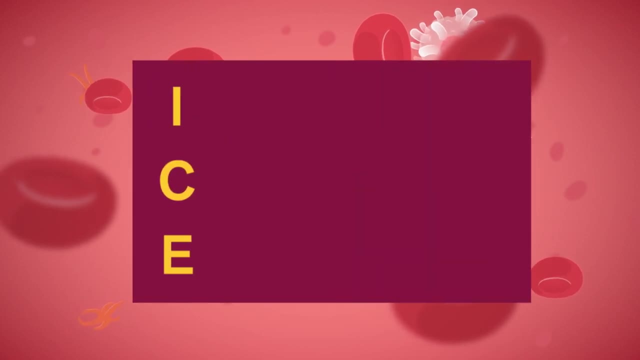 carbonic acid to H+ and bicarbonate, which successfully regulates our pH. We don't have time here to go into all the details of these interactions, but making a table to calculate the ice or initial change in equilibrium concentrations in a reaction. 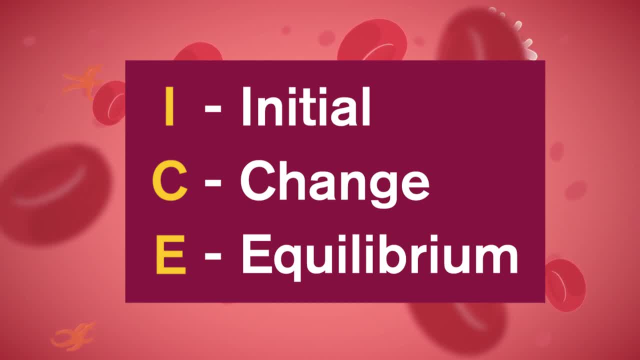 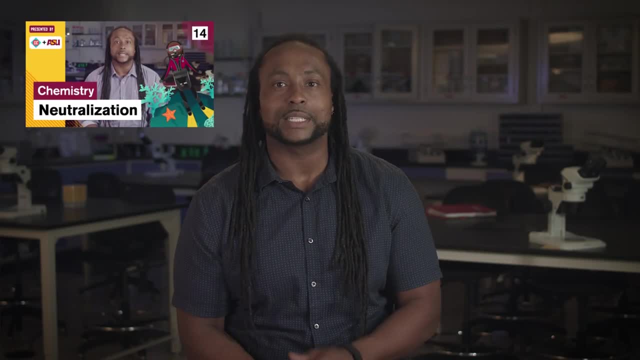 is another way chemists solve more advanced buffer problems. We're going to stick to the basics for today, though Let's move on to strong acid and base reactions. In the last episode, we learned that when strong acids and strong bases combine and 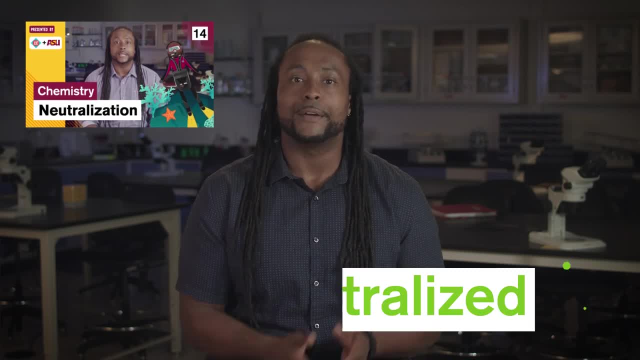 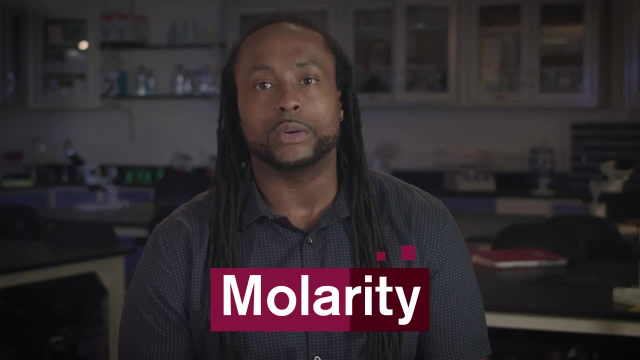 there are no H+ or OH- ions left over. they're fully neutralized, since they form neutral water and salt. If we want to neutralize an acid or base properly, we also need to know its concentration in moles per liter or molarity. 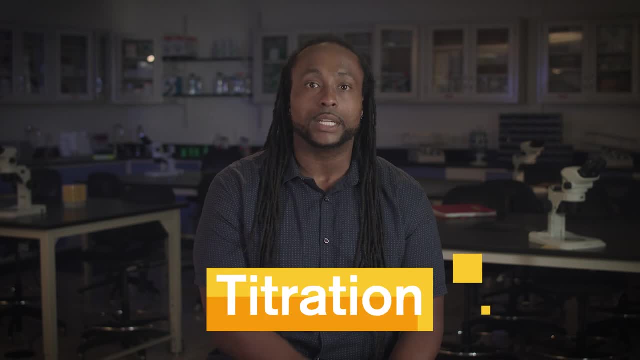 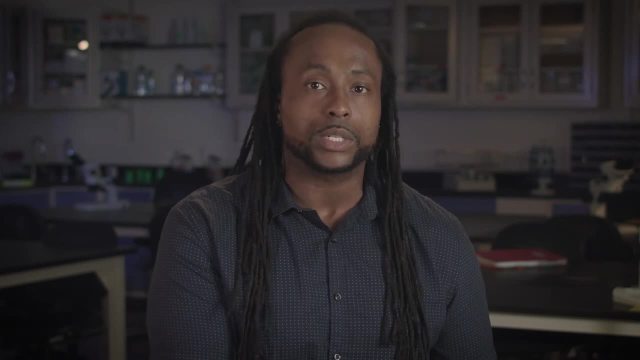 But if we have an unknown concentration of the acid or base in our reaction, we have to perform a titration. This is where we would slowly add an acid or base with a known concentration to our unknown solution to determine how much is needed to neutralize. 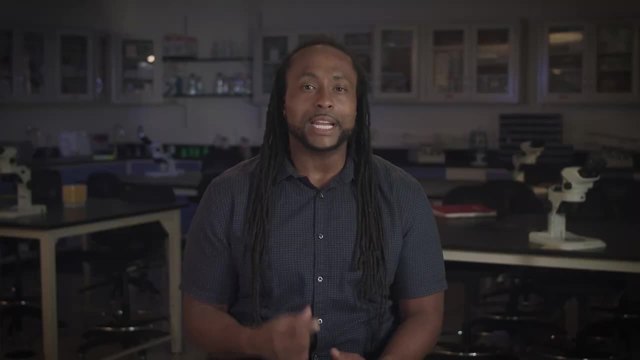 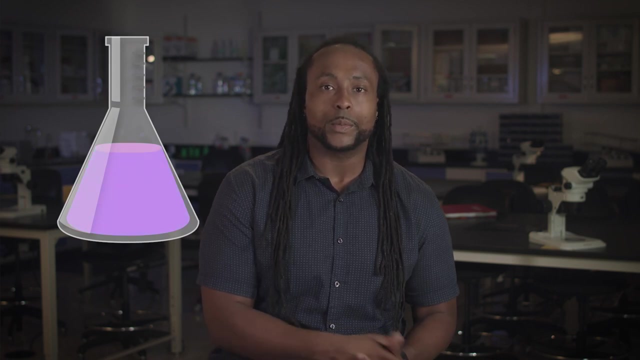 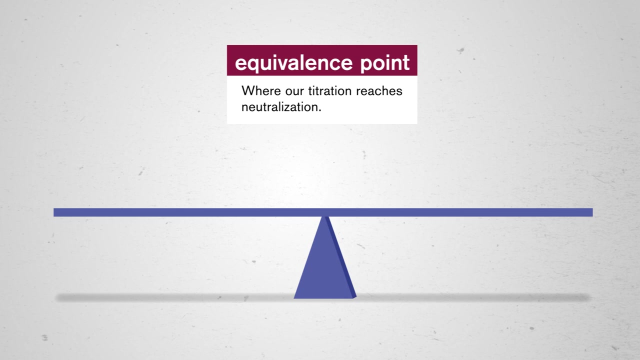 From there we can figure out its concentration. We add a color indicator chemical to our unknown solution that will change colors once our solution has neutralized. We call the point where the color changes and stays that color, the end point At our equivalence point, which is exactly where our titration reaches neutralization. 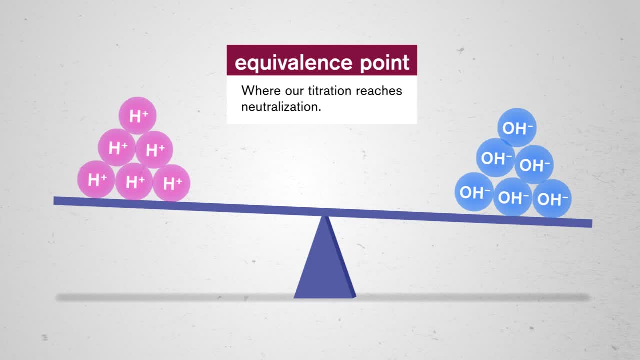 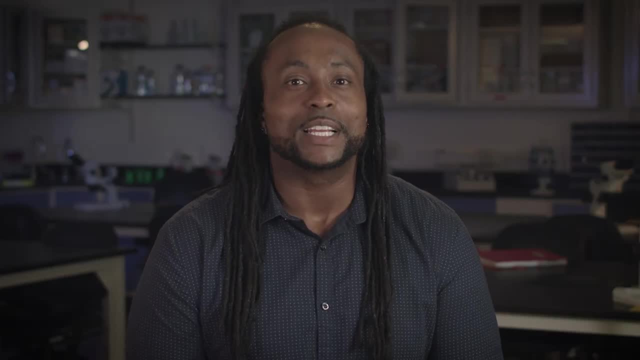 the solution will have the exact same amount of H+ and OH- ions and the pH will always be 7.. The equivalence point and the end point are not the same. Usually, the color indicator won't turn until it's neutralized. 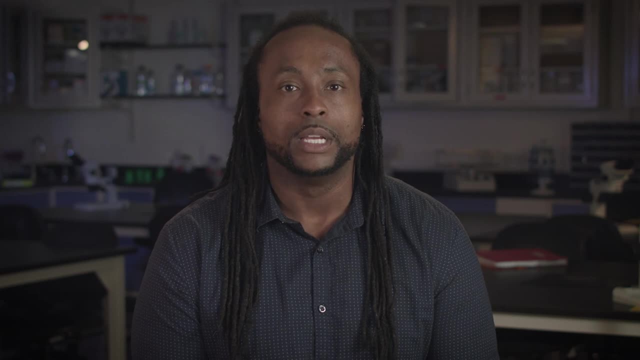 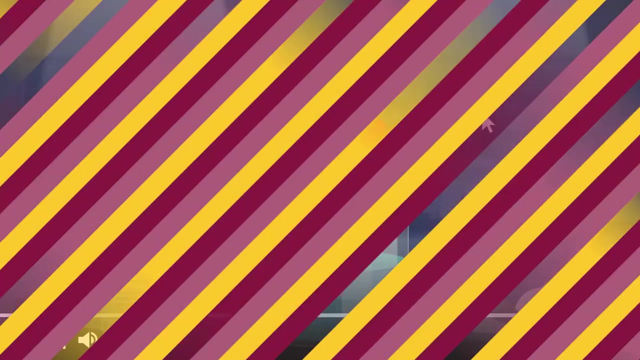 It won't turn until after the solution's passed its equivalence point. so it's more precise to use equivalence points for calculating concentrations. Let's try a titration with hydrochloric acid and sodium hydroxide- a strong acid and strong base on test tube. 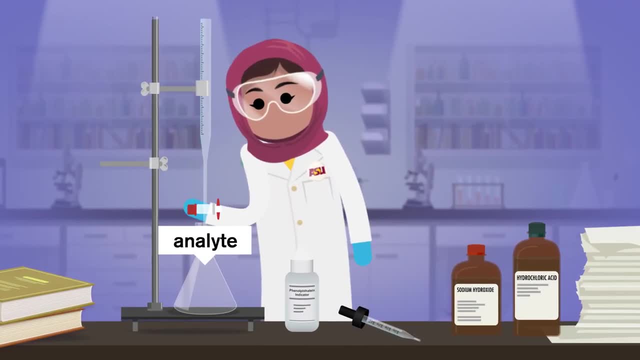 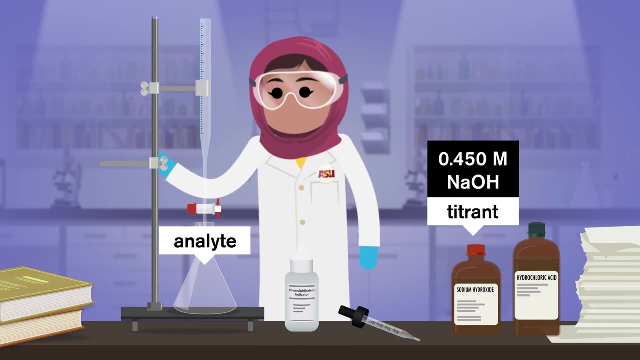 We've got 21 milliliters of acid, which is our analyte. the substance with an unknown concentration, Sodium hydroxide, is our titrant, meaning we do know its concentration at 0.450 molar. Our titration will reveal the titration value at 0.450 molar. 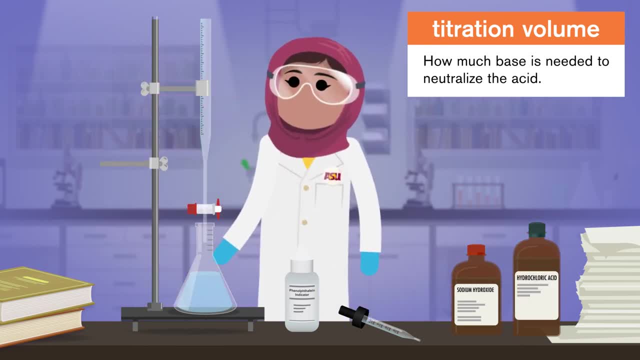 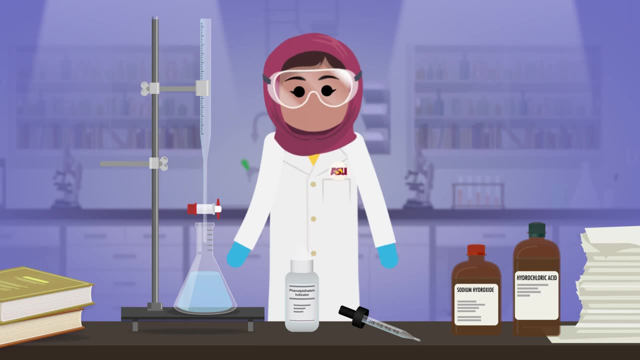 We'll measure the base volume, or how much base is needed to neutralize the hydrochloric acid. First we'll add a bit of phenolphthalein, a color indicator, to the hydrochloric acid, and place it under our burette setup. 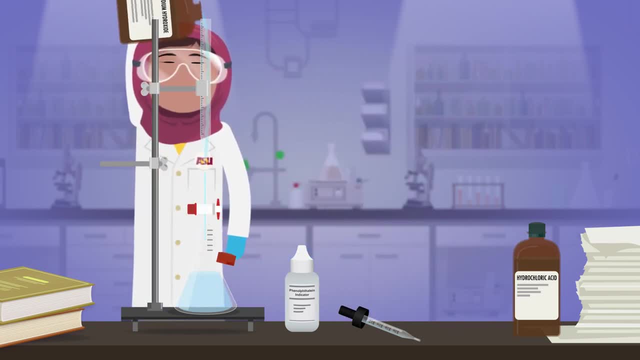 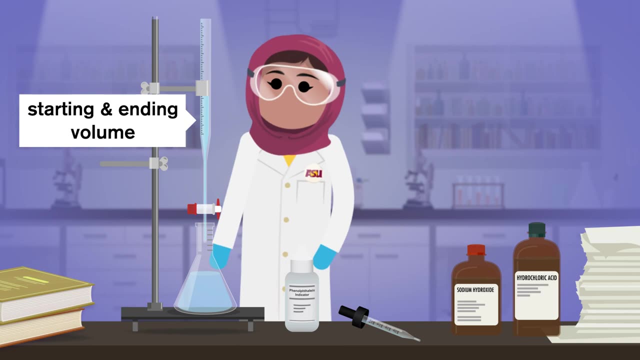 Then we'll pour a bunch of sodium hydroxide into the closed burette. We need enough to fully complete the titration and not run out too early. The burette will measure the starting and ending volume of our base. Next we'll open the burette and slowly add drops of sodium hydroxide into our acid. 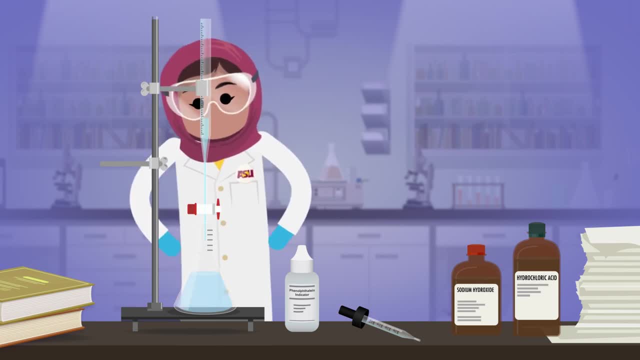 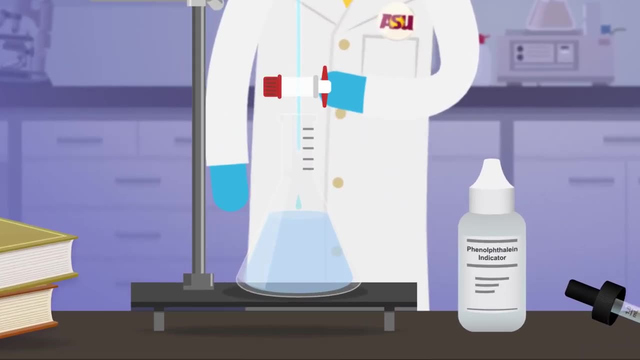 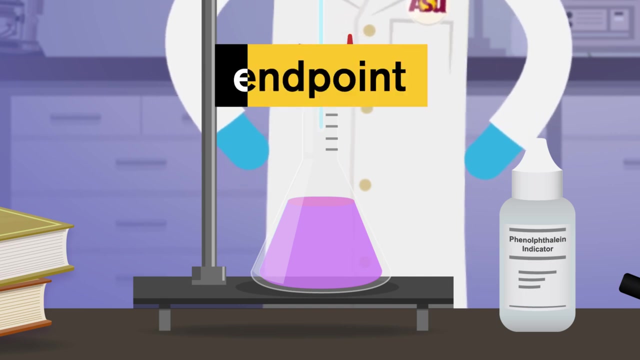 stirring to let the two solutions mix properly To flash between clear and pink. we have to be careful not to add too much base too fast. Usually chemists will go one drop at a time, trying to be as precise as possible. Once the acid turns pink and stays pink. this is the endpoint and the end of the titration. 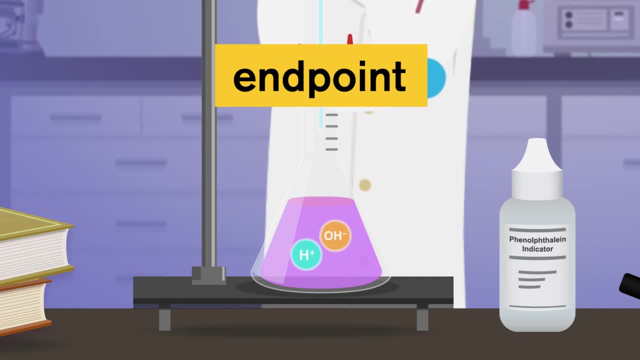 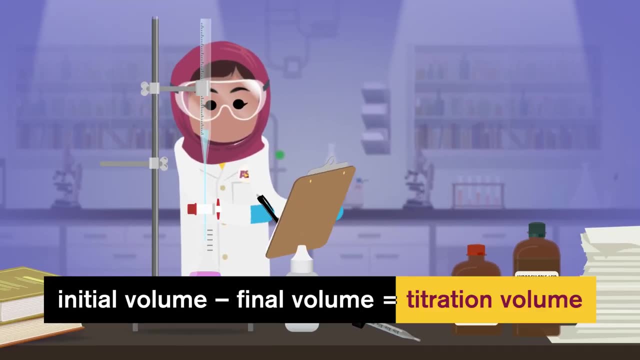 All the acid's H-plus ions have been neutralized by the OH-minus ions from the base and we're left with some super cool pink water and sodium chloride. Last thing: We need to subtract our final volume from our initial volume to find out how much sodium. 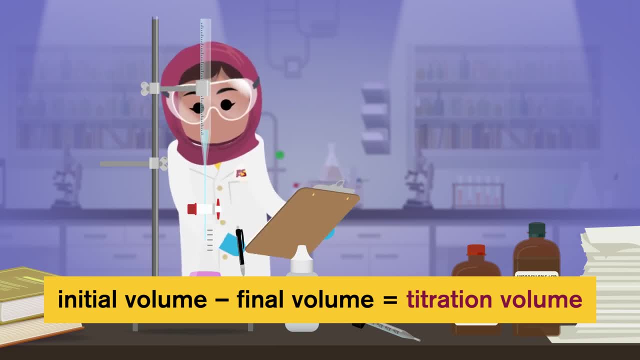 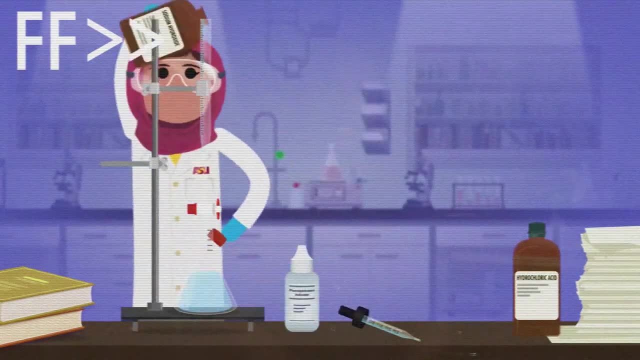 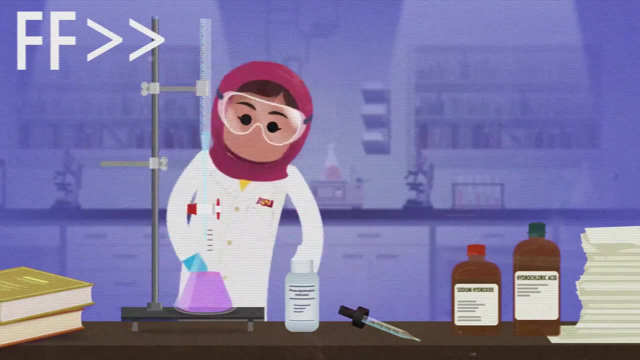 hydroxide is left To find out the amount of sodium hydroxide we needed to neutralize the acid. this is our titration volume To get the exact amount needed to reach our equivalence point and not just the endpoint. chemists usually perform the same titration multiple times, averaging the titration volumes. 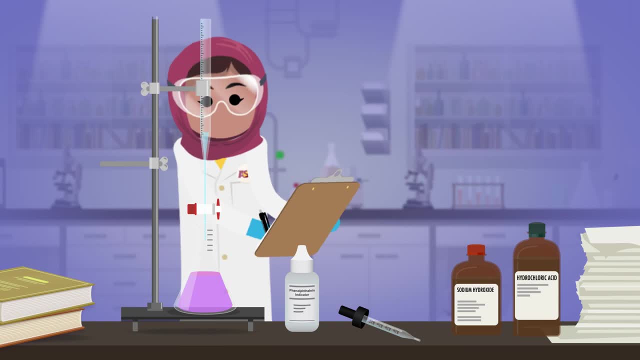 together to get a more accurate result. Let's assume we've done this and for this experiment we needed 47 milliliters to get to the equivalence point of our titration. Now that we know both the volume and molar concentration of our sodium hydroxide, we're 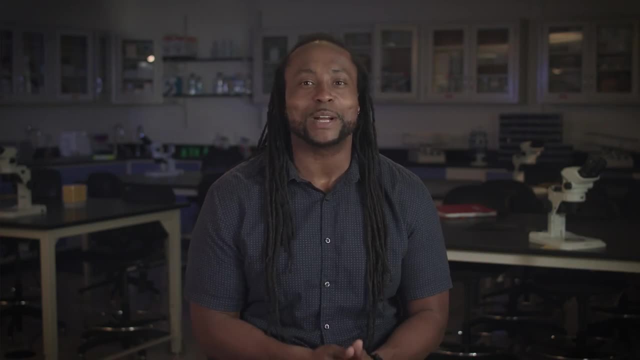 going to be able to calculate the amount of sodium hydroxide we need to neutralize the acid. Since we know the titration concentration of our sodium hydroxide solution and we know the initial volume of our hydrochloric acid solution, our next step is to calculate the 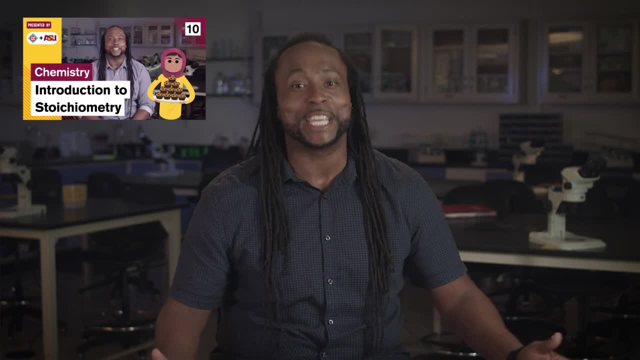 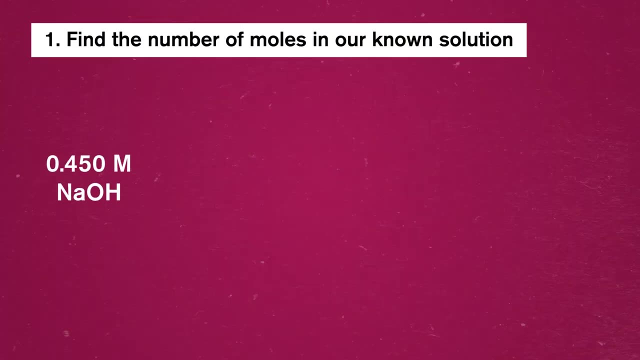 hydrochloric acid mystery concentration using stoichiometry. To get to our mystery concentration we'll perform three steps. We'd first need to take our molarity of sodium hydroxide at 0.450 moles per liter and multiply it by its titration volume to end up with moles. 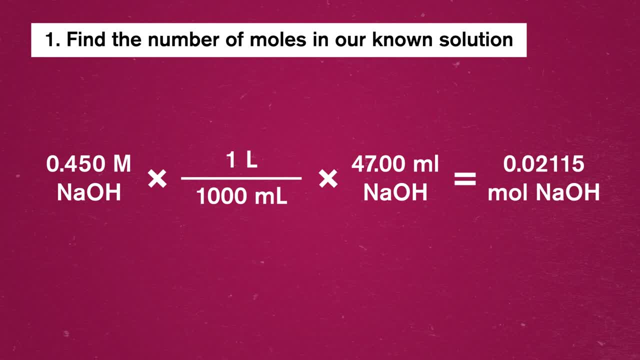 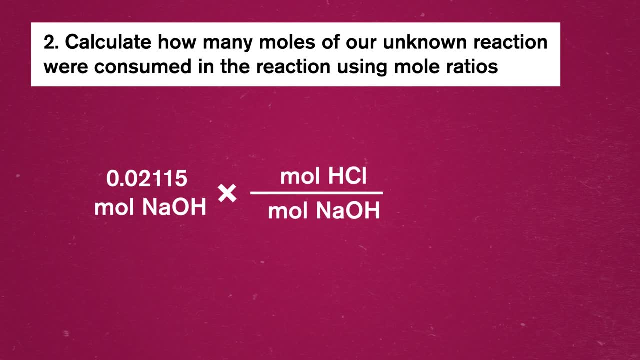 Since our volumes are in milliliters, we'll need to convert to liters along the way. Gotta love the metric system. It makes this a lot easier. Step two is converting moles of sodium hydroxide to moles of hydrochloric acid with a mole ratio. 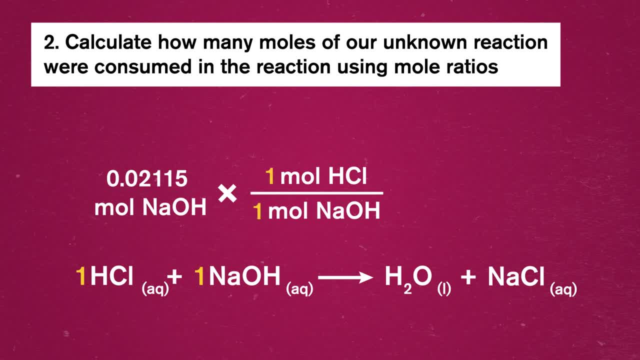 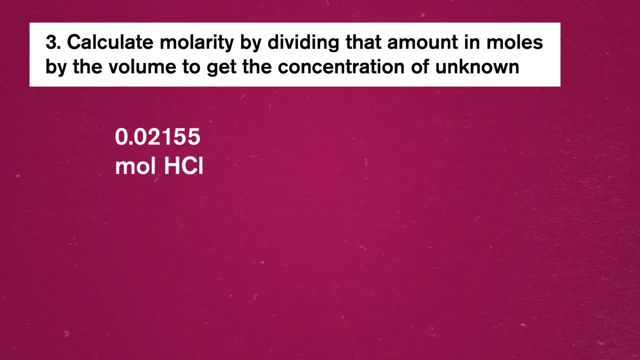 In this case, our ratio is 1 to 1, so we end up with 0.0215 moles of hydrochloric acid consumed in the reaction. Our last step is to take that amount of moles and divide it by our given starting volume. 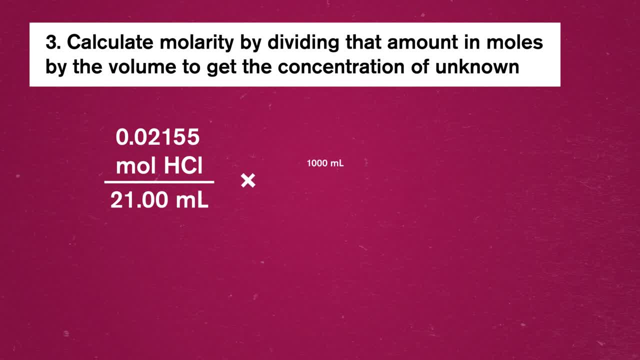 of hydrochloric acid. to get our molarity, We'll need to convert from milliliters to liters. here too, Thanks to our titration and a little bit of math, we're now able to calculate the ratio of hydrochloric acid to moles.